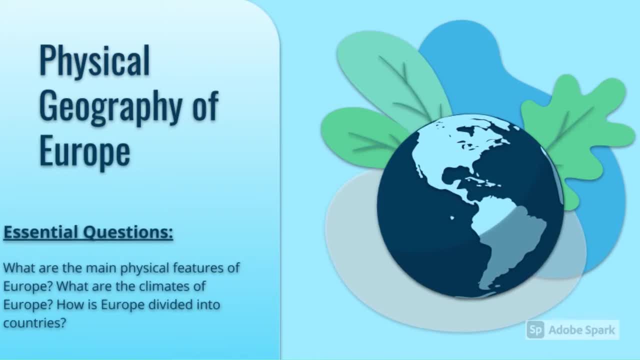 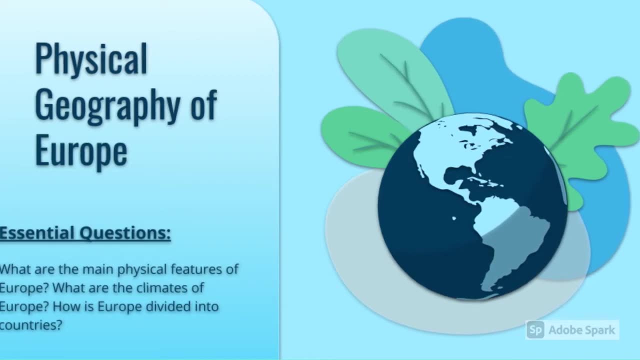 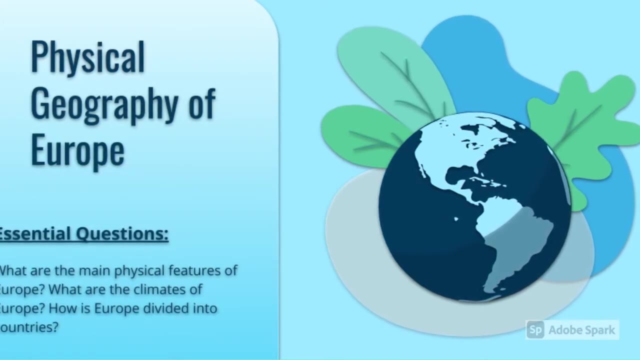 So we're going to start with the physical geography of Europe. We have three essential questions. The first one is: what are the main physical features of Europe, What are the climates of Europe, And how is Europe divided into countries? Let's find out. 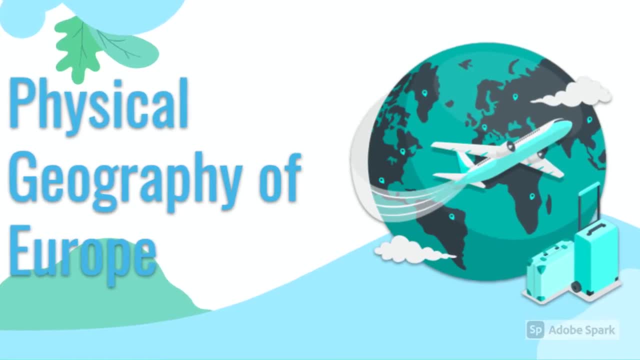 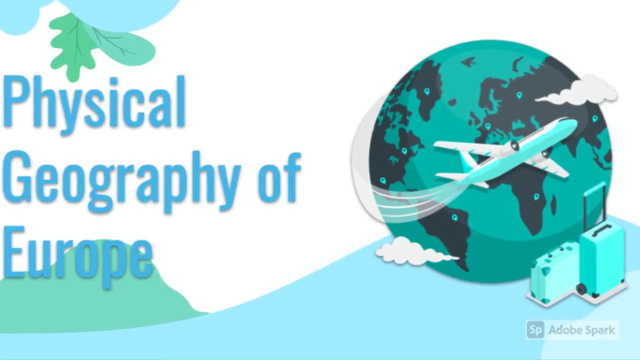 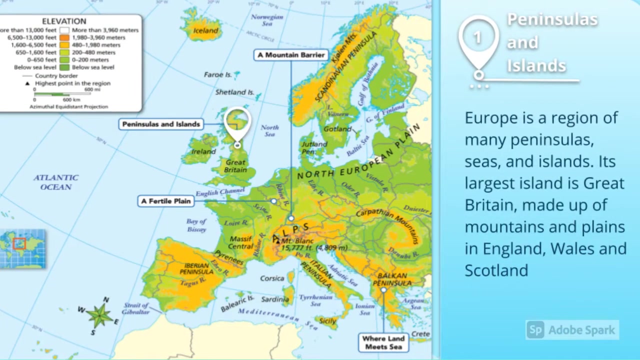 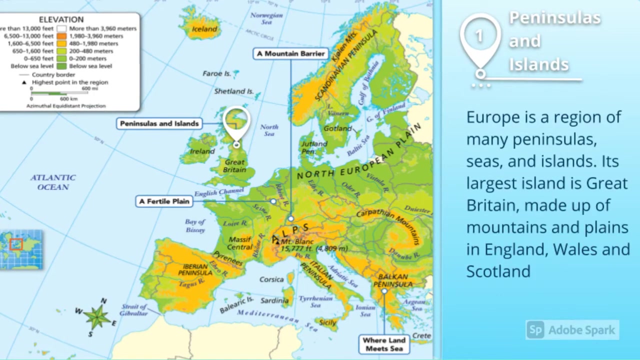 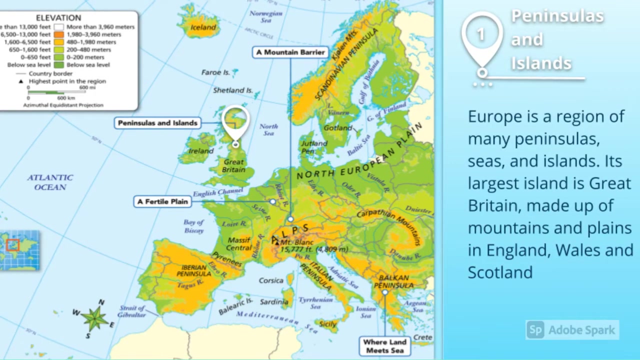 The first step in answering our questions is going to be to talk about the physical geography of Europe. We're going to be using a physical map and talking about landforms that are prevalent in Europe and around the world. The first landform that we will be talking about is a peninsula. A peninsula is a piece of land that juts out into the ocean or into water. It has water on all sides, except for one place where it connects to a mainland. An island is surrounded by water on all sides. 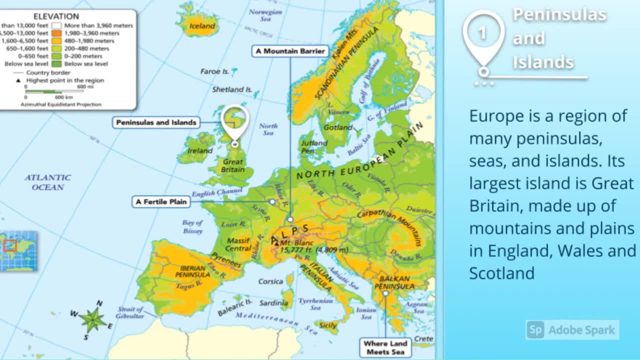 Europe is a region of many peninsulas, seas and islands. Europe is a region of many peninsulas, seas and islands. Its largest island is Great Britain, made up of mountains and plains in England, Wales and Scotland. 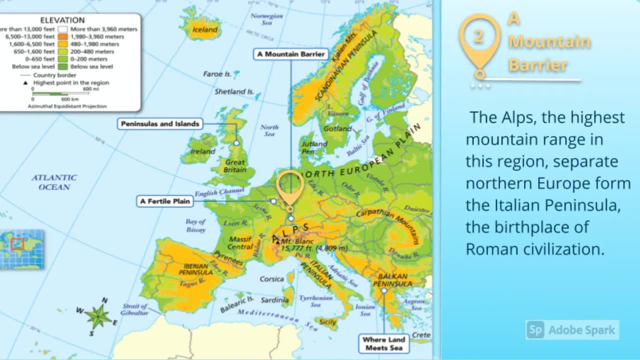 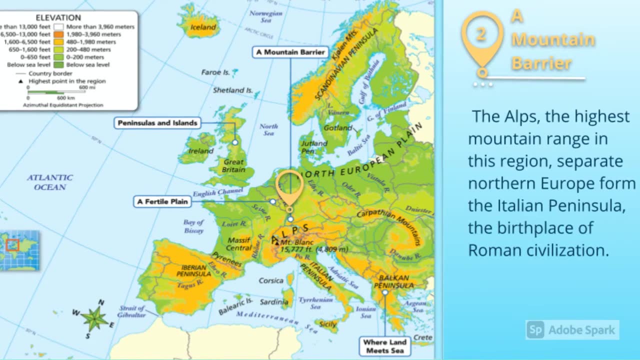 Right through the heart of Europe, there is a mountain range called the Alps. This is called a mountain barrier. The Alps is the highest mountain range in the region and it separates northern Europe from the Italian peninsula, which is the birthplace of Roman civilization. 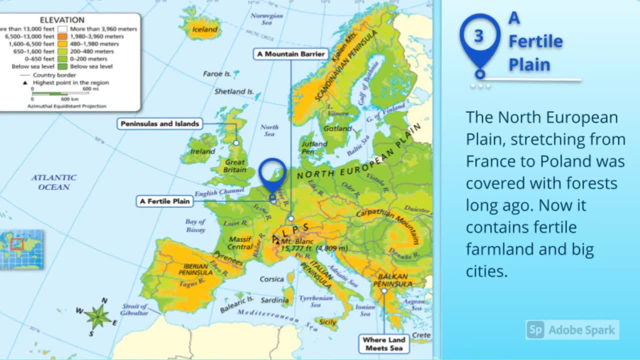 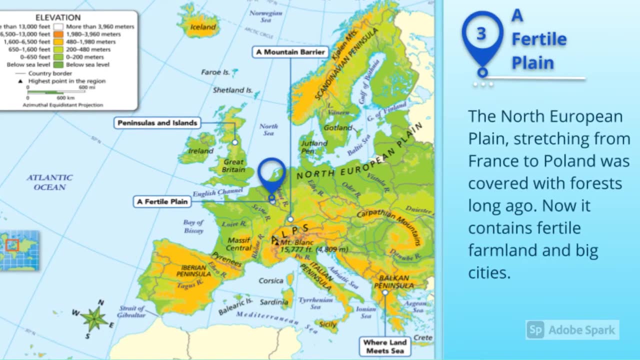 Also in Europe. the big area in the heart is a good place for farming. We call this a fertile plain. The northern European plain stretching from France to Poland was covered with forests long ago. Now it contains fertile farmland and big cities. 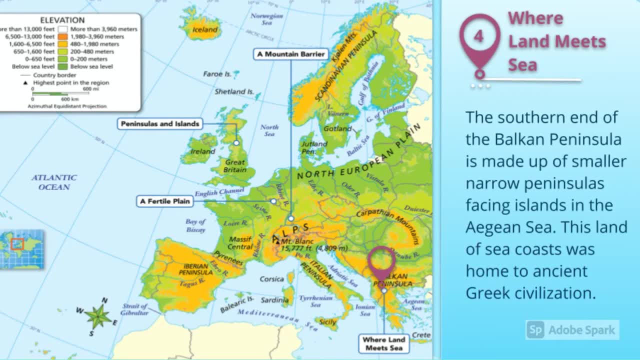 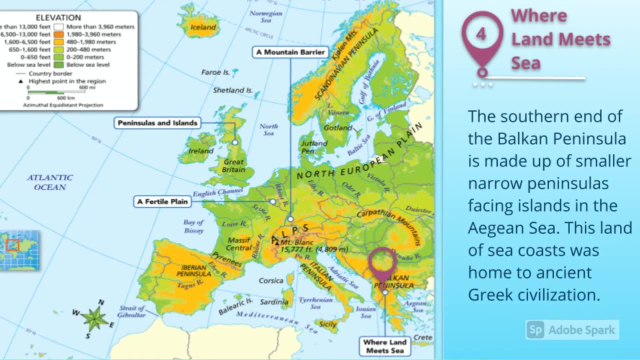 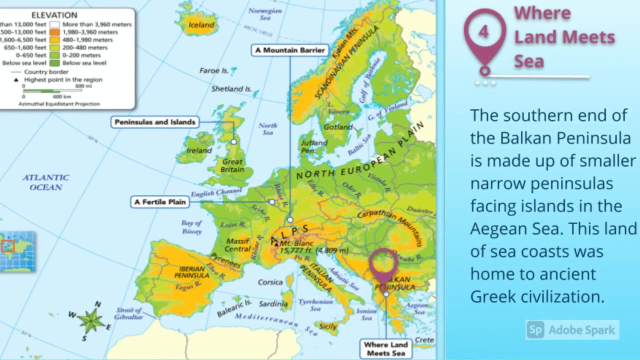 Down in southern Europe we have a place where land meets the sea. This is the southern end of the Balkan peninsula and it's made up of smaller, narrow peninsulas facing islands in the G and C. This land of sea coasts was home to ancient Greek civilization. 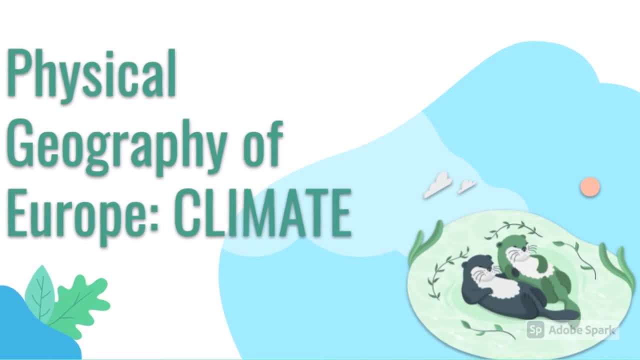 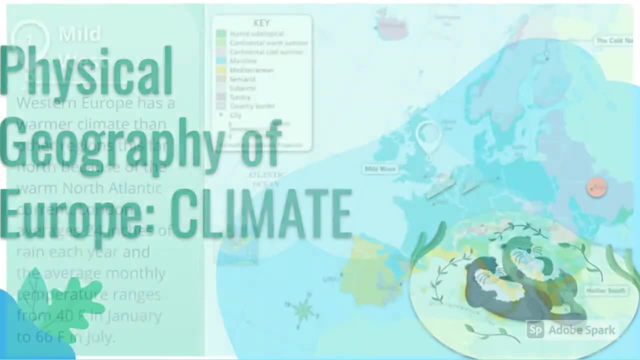 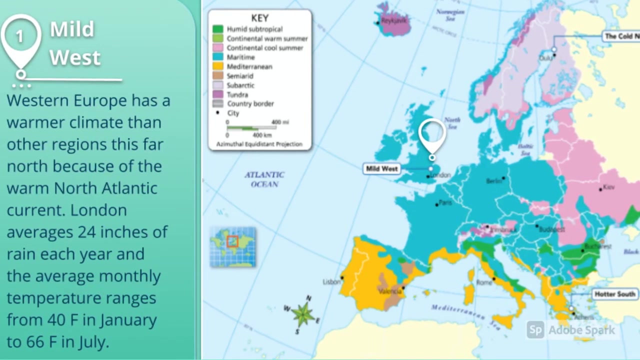 Our second essential question deals with Europe's climate. We're going to be using climate maps in order to learn about the primary climates that can be found in Europe. Europe is a large continent with a lot of different climate zones. Overall, we can summarize: 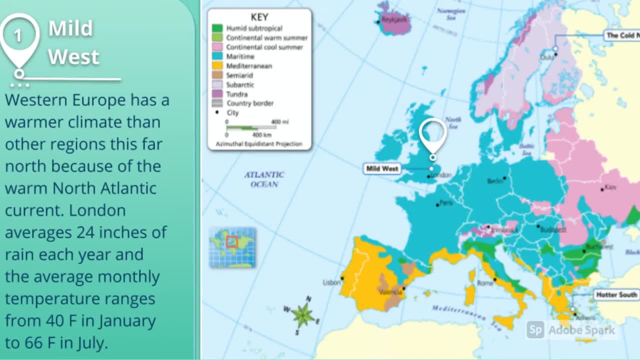 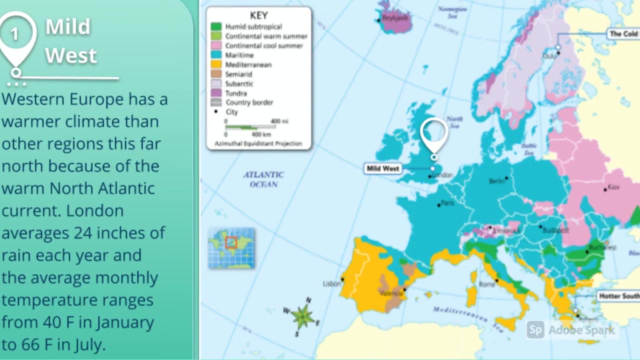 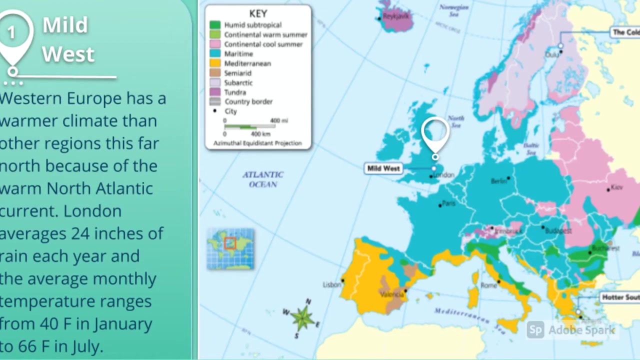 these into three chunks. Chunk one is the mild west. Western Europe has a warmer climate than other regions this far north because of the warm North Atlantic. current London averages 24 inches of rain each year and the average monthly temperature ranges from 40 degrees in January to 66 Fahrenheit in July. 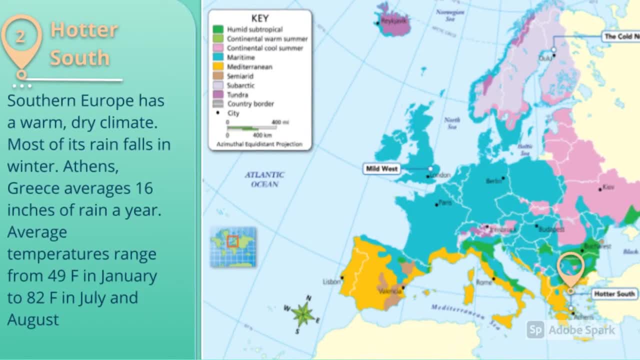 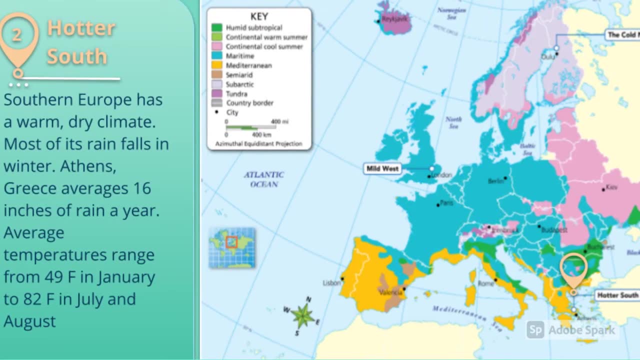 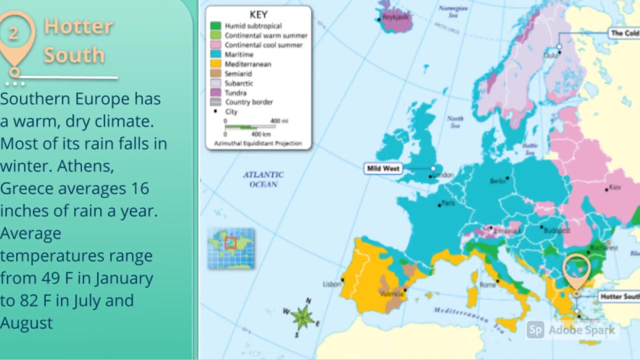 As we get closer to the equator, we reach the hotter south. Southern Europe has a warm, dry climate. Most of its rain falls in winter. Athens, Greece, averages 16 inches of rain a year. Average temperatures range from 49 degrees Fahrenheit in January to 82 degrees. 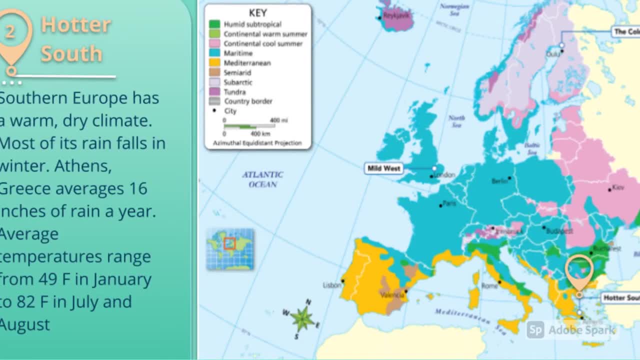 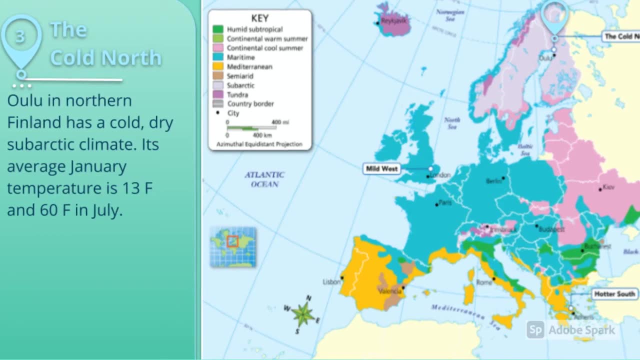 Fahrenheit in July and August Much warmer than the north. The farther north we go, the colder it gets And finally we'll reach the cold. north, Oulu and northern Europe have a warm and dry climate. Southern Europe has a warmer and. 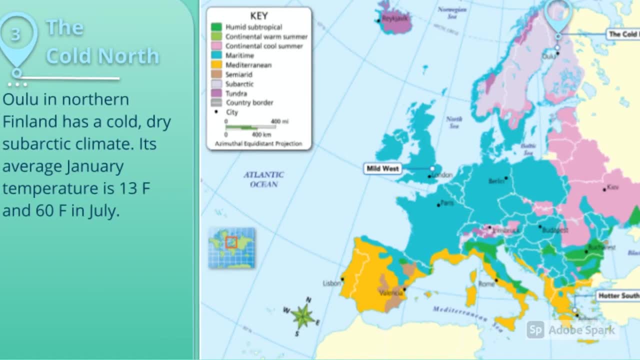 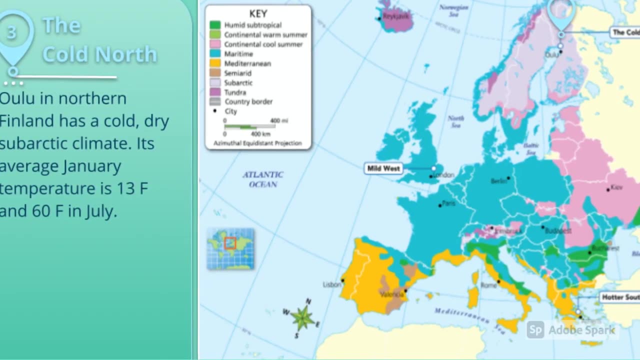 warm climate than other regions. this far north Western Europe has a warmer and warmer. northern Finland has a cold, dry sub-Arctic climate. That means it's just below the Arctic Circle. Its average January temperature is 13 degrees Fahrenheit and it reaches 60 degrees. 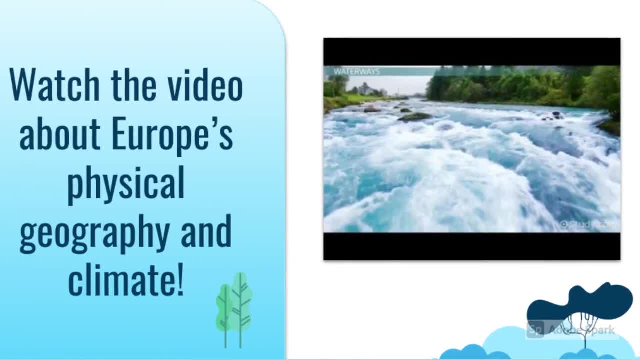 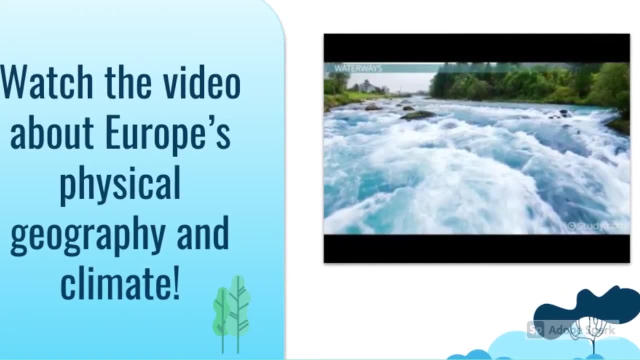 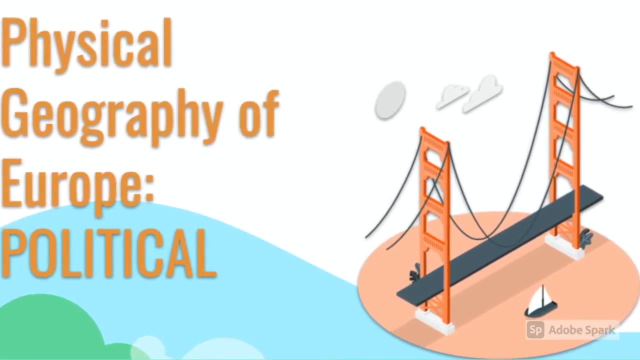 Fahrenheit in July. We're going to pause a little bit and we're going to watch a video about Europe's physical geography and climate. Our final essential question discusses how boundaries are drawn in Europe. We're going to be looking at political maps to answer these questions. 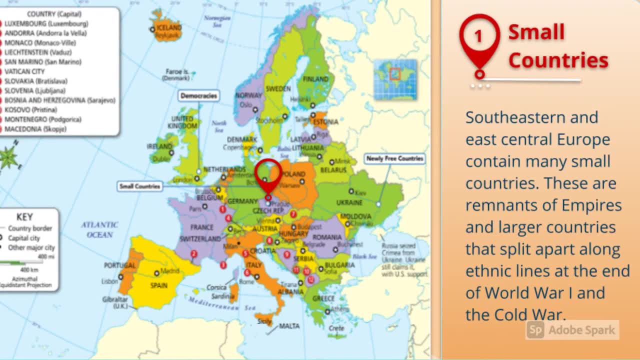 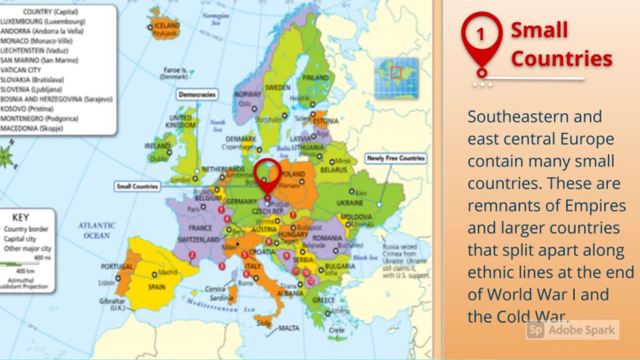 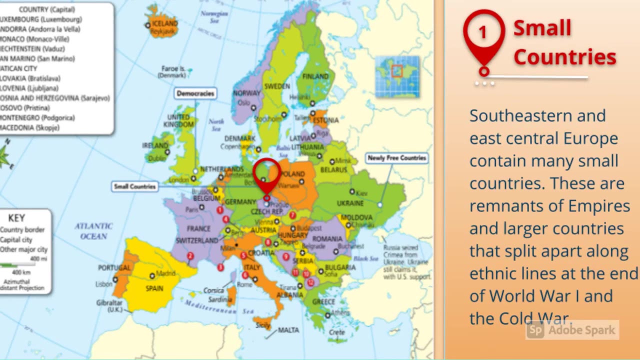 One type of political boundary you'll see in Europe are small countries, and southeastern and east-central Europe contain many small countries. These are remnants of empires and larger countries that split apart along ethnic lines at the end of World War I and the Cold War. 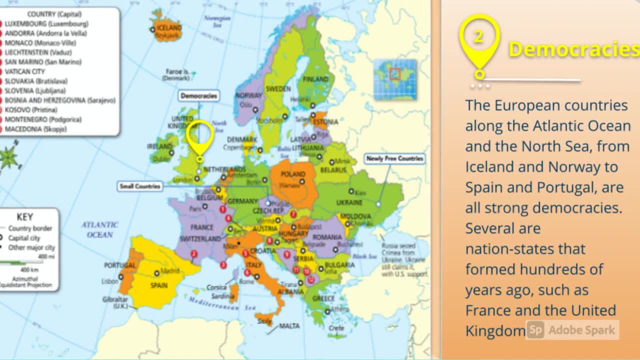 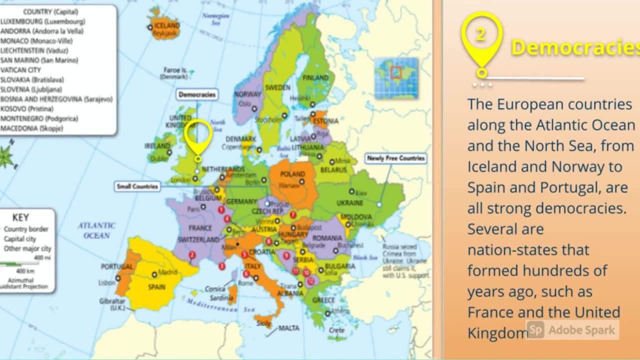 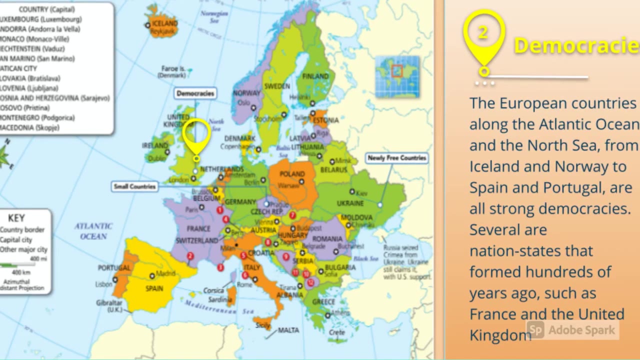 Also in Europe you'll find quite a few democracies. The European countries along the Atlantic Ocean and the North Sea, from Iceland and Norway to Spain and Portugal, are all strong democracies. Several are nation-states that formed hundreds of years ago, such as France and the. 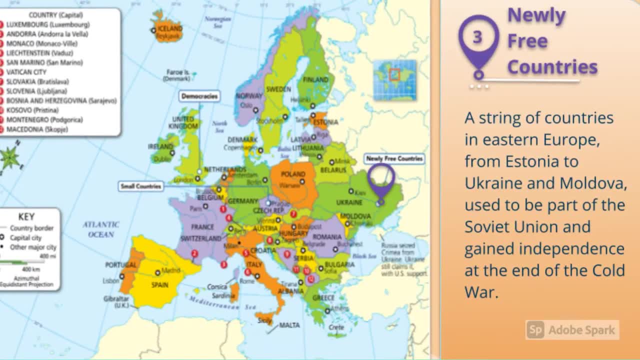 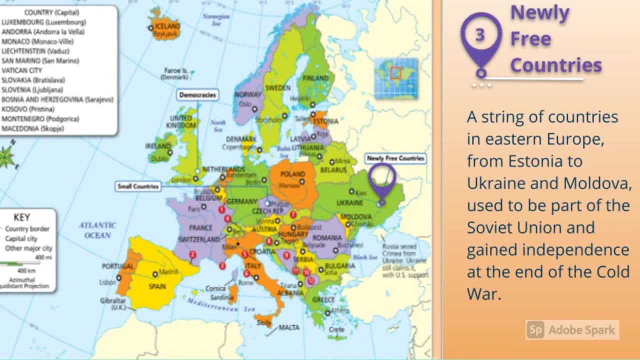 United Kingdom. Finally, we have some new kids. These are the newly free countries. A string of countries in Europe are part of Europe, including the Soviet Union, Poland and Culture. Click the link below to learn more about the names of the countries.